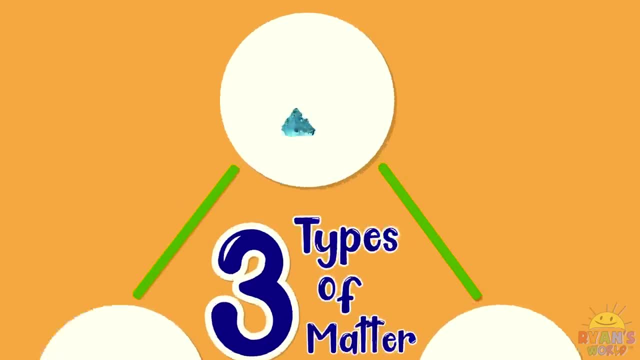 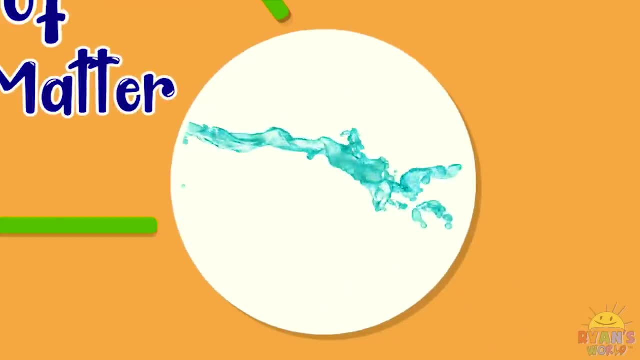 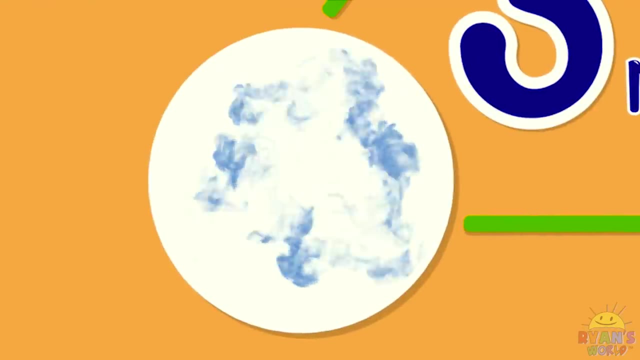 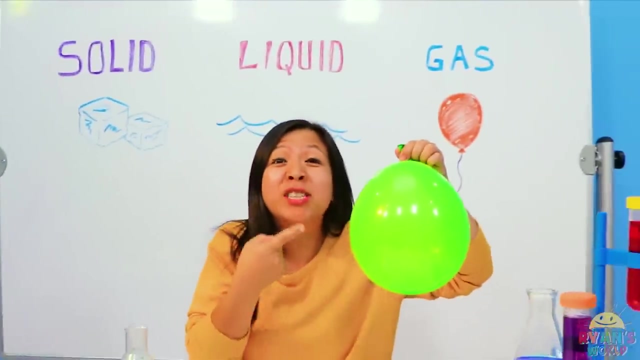 And there are three types of matter: Solid, Like this ice- Oh, cold cold. Liquid, Like this watercolor. Or gas- Oh, hold on, There we go Now. the balloon is full of air, which is gas inside. 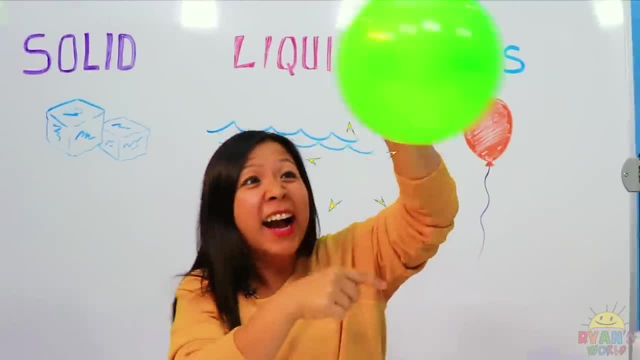 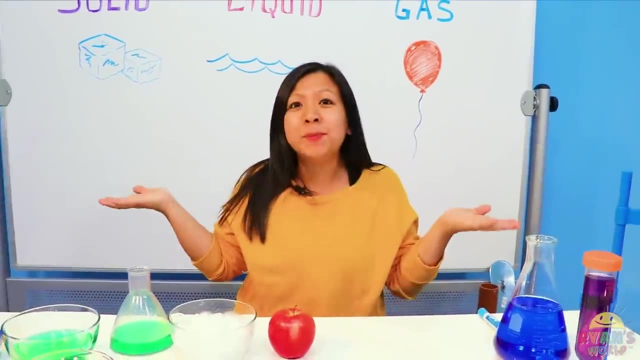 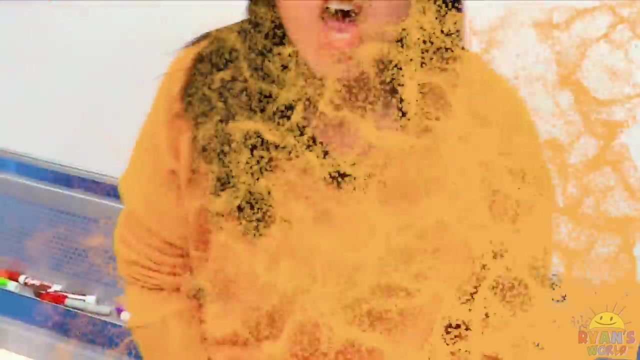 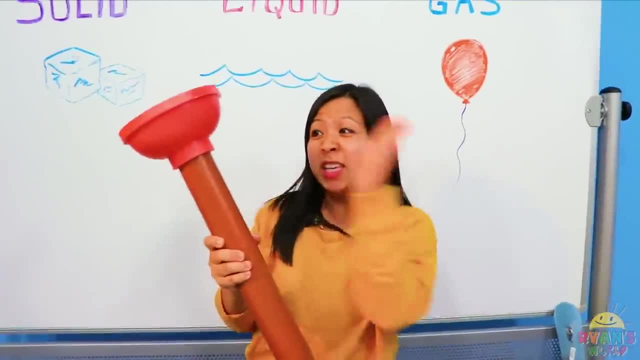 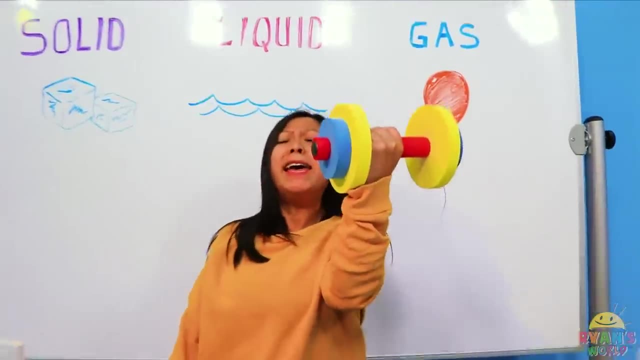 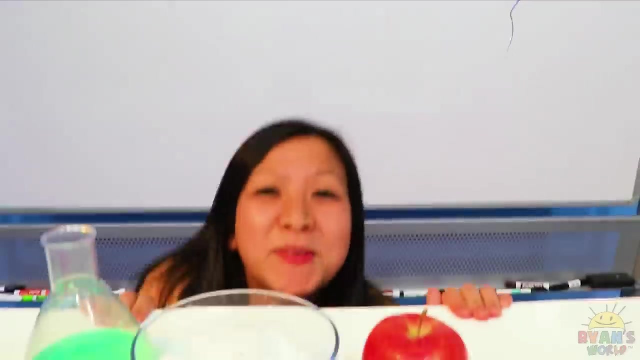 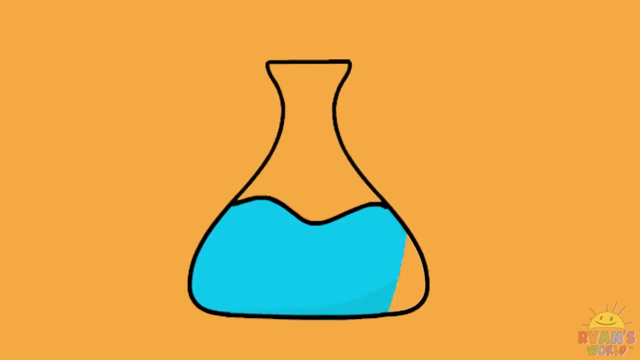 This is also a solid, Right. It keeps its shape and volume And this is also a solid, Solid. Solid, the same shape and volume, I'm okay. Liquids, however, have particles that are free to move around. It keeps the same volume, but different shapes. 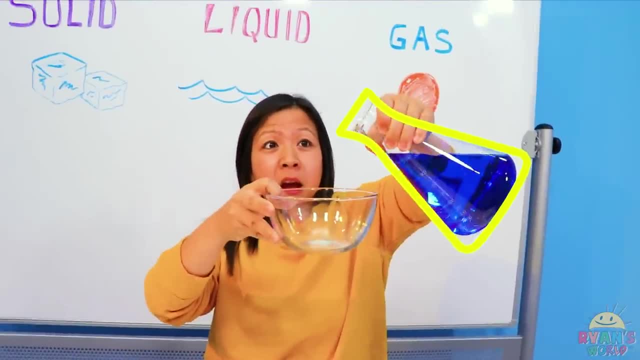 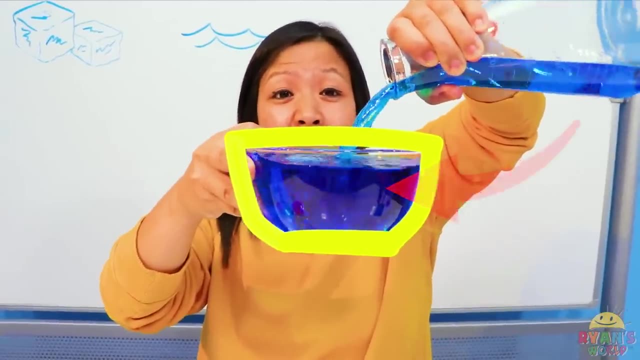 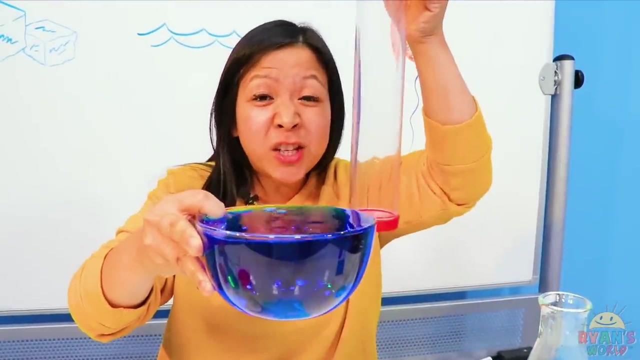 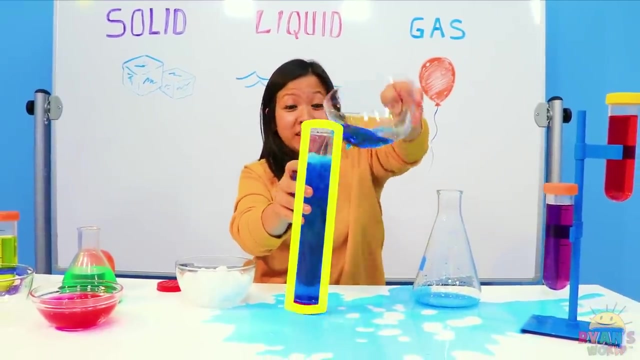 For example, this liquid here. look what happened. See, it keeps the shape of the container, but it's the same amount of volume. Now let's put the liquid into a different shaped container. This is the shape of a bowl, And now this is the shape of this cylinder. 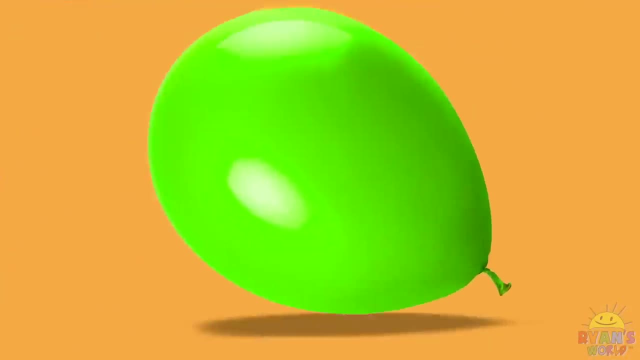 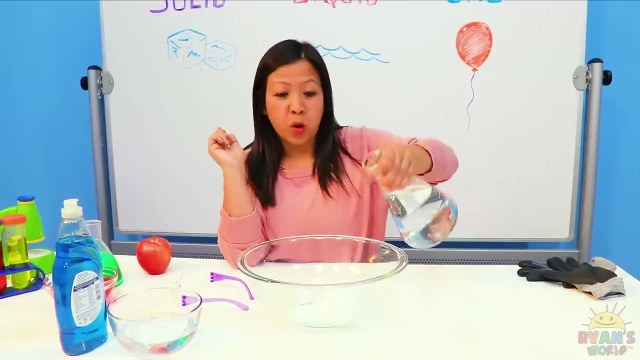 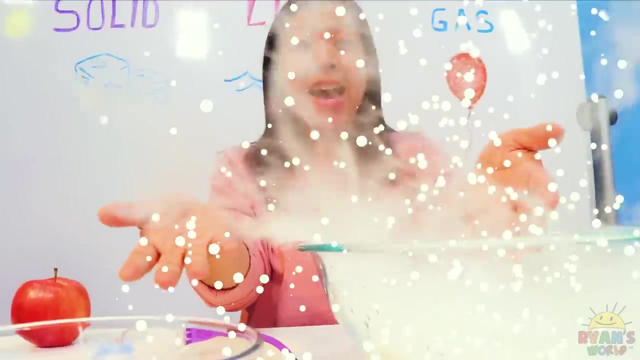 Gas have particles that are so loose they have no definite shape or volume. So this- I have dry ice and I'm gonna mix it in with water And look, it produces carbon dioxide Gas. it just goes everywhere, filling up the whole room. 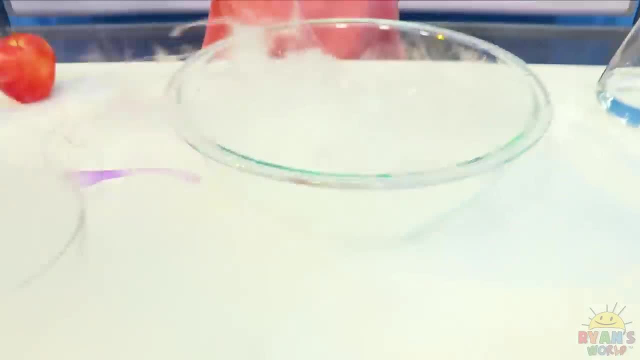 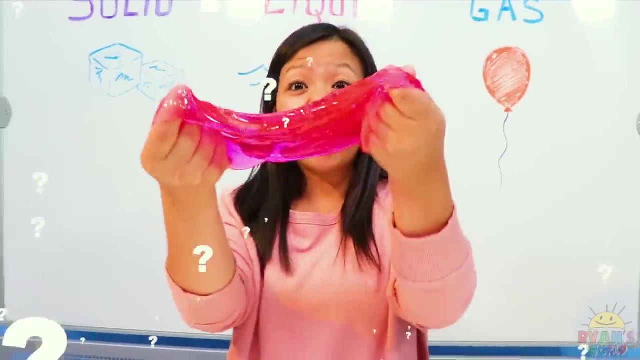 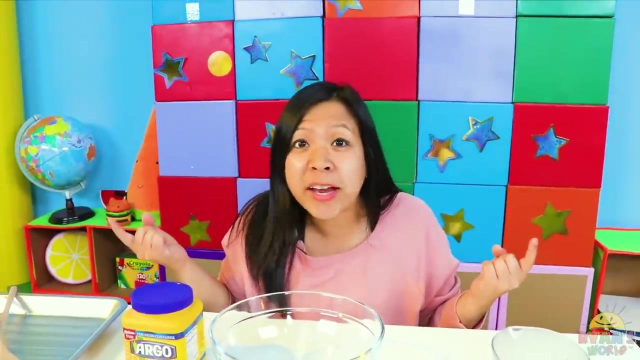 Whoa. look at the gas flow. But what happens with things like slime? Is this a solid or is it a liquid? Before we explain what is slime, let's make our own special kind called oobleck. All you need is cornstarch, a scoop coloring. 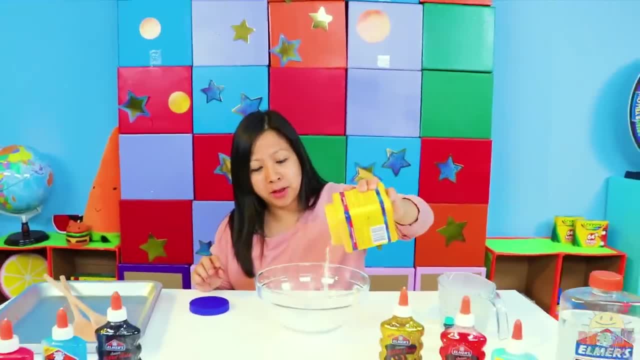 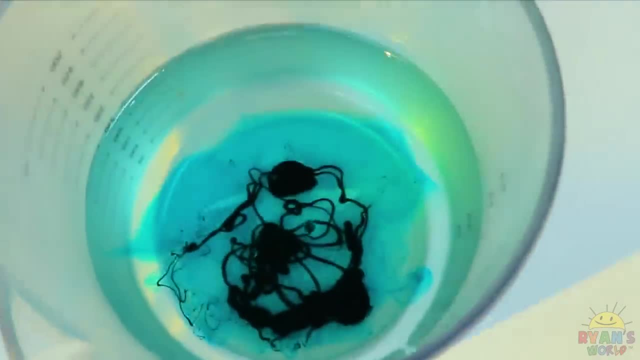 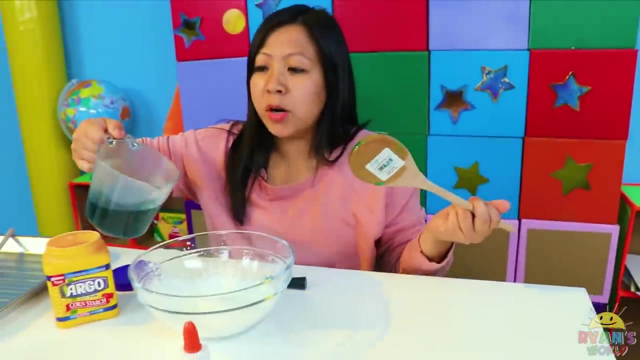 and a spoon. And what's inside that spoon Water? Pour it inside a bowl. Let's make our water color green. That's pretty. Get a spoon, agitate it, then pour it into our cornstarch, Mix it up. 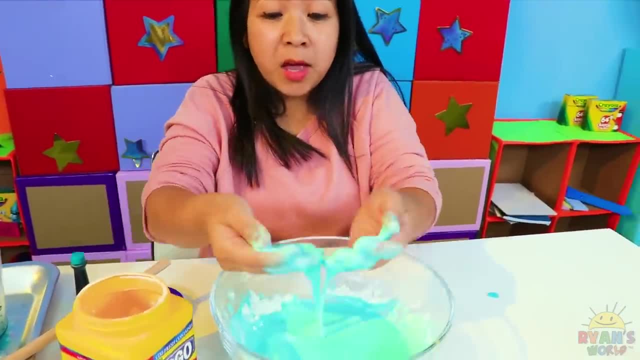 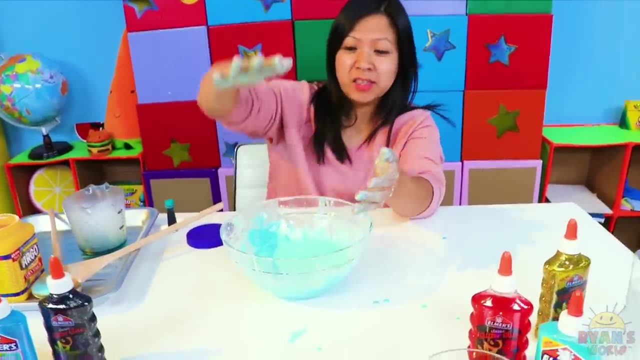 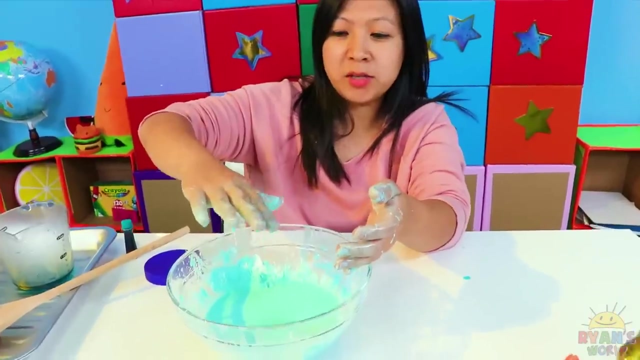 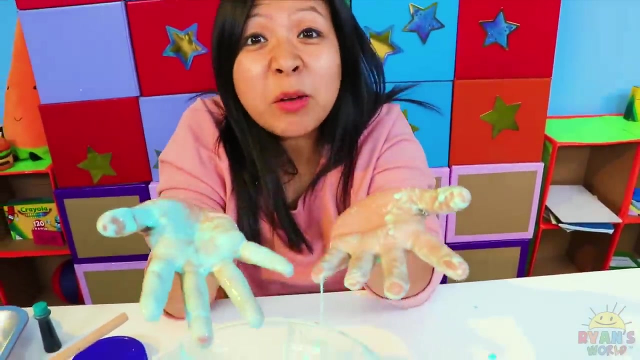 Now this is really cool because, look, if you pick it up, it looks like a liquid. see, liquid. but what happened if you tap it like this? whoa, it was hard like cement. again one, two, three. what if I do it slowly? it's a liquid. what's going on? so? 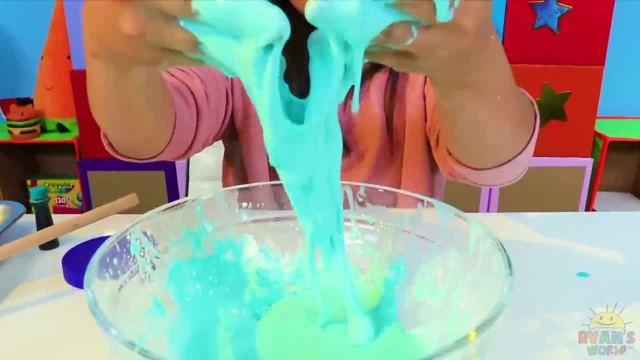 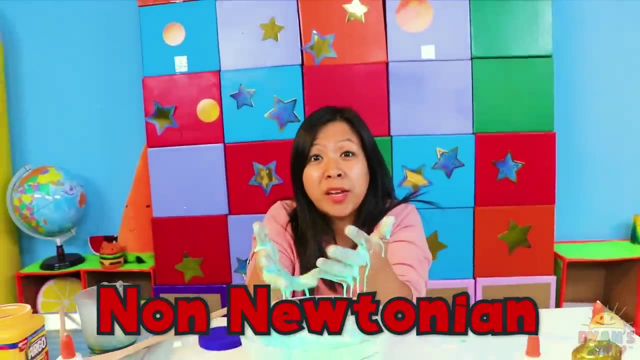 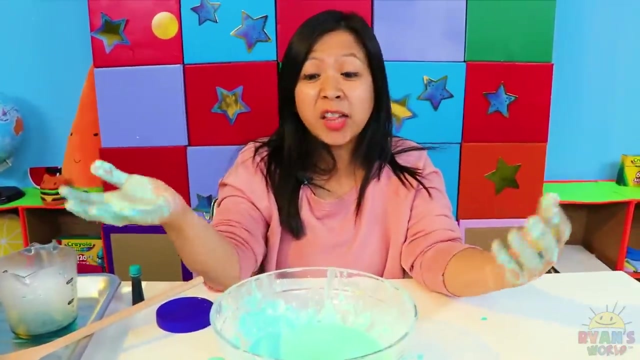 it's slime like oo black. is this a solid or a liquid? well, this is a special kind. it's called non-newtonium liquid. but what is a non-newtonium liquid? well, it can behave as a solid when pressure is applied like this, or it could behave. 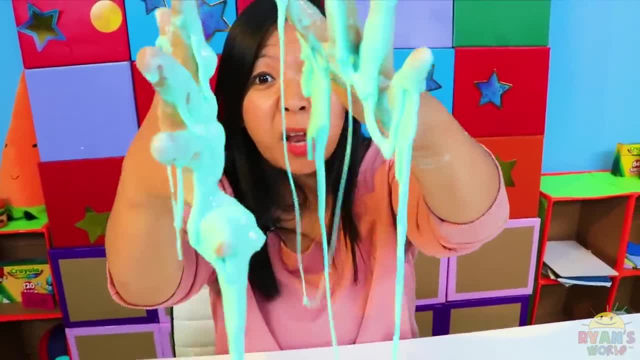 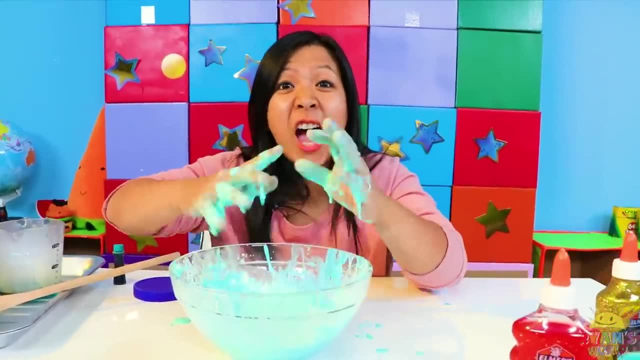 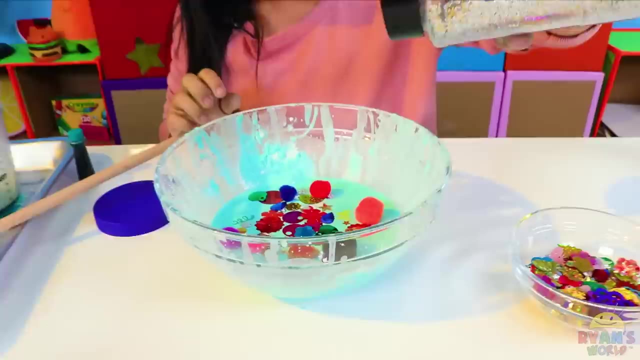 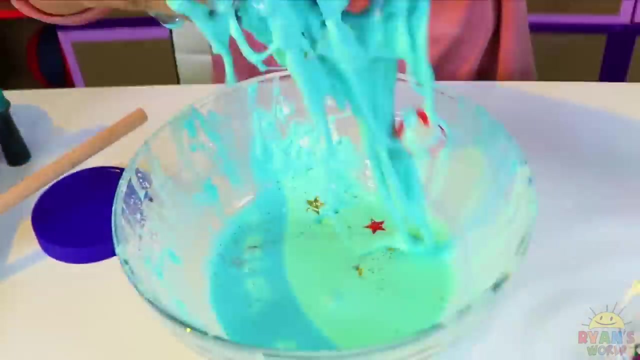 like a liquid when pressure is not applied. pretty cool stuff, huh, I have an idea. why don't we mix it up and add glitter and other things to our old black? some pom-poms, glitter there. mix it up. oh look how cool this looks. wow, there it is. 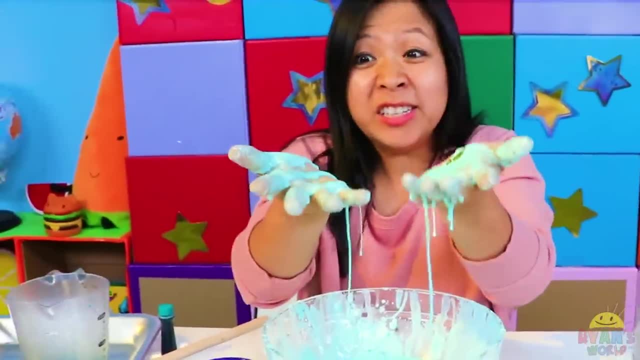 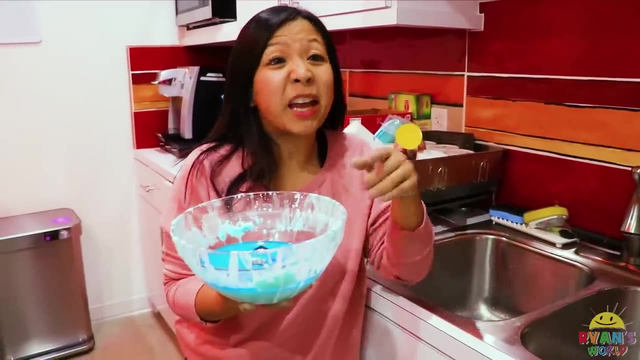 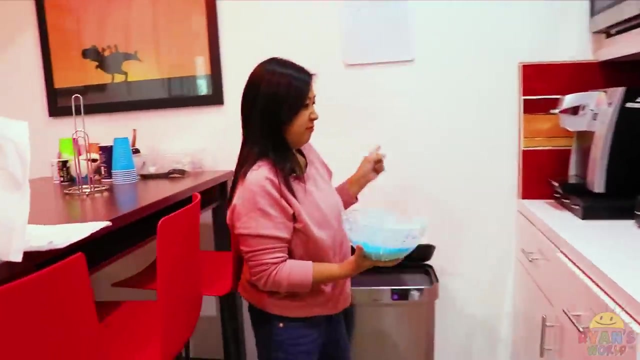 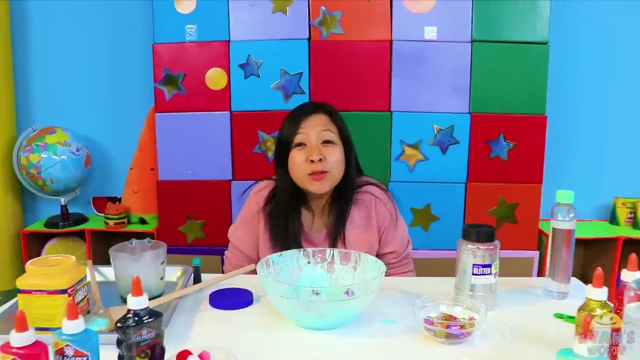 your own non-newtonium liquid. is it a solid or is it a liquid? both? when you're done playing with your old black, do not pour down the sink, or else it might clog the sink. you can either pour it in the trash or you can save it in the ziplock bag so you can play with it for later. so to 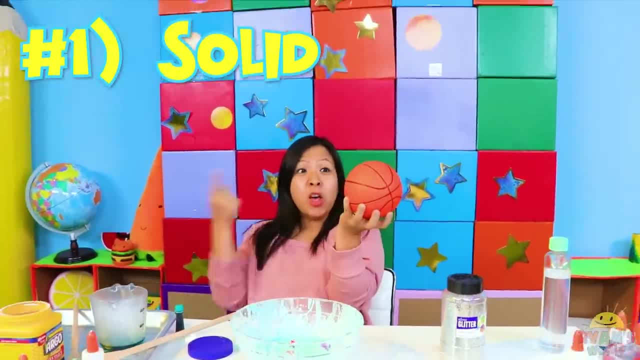 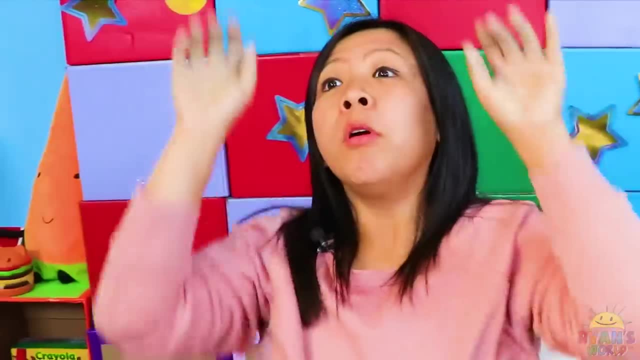 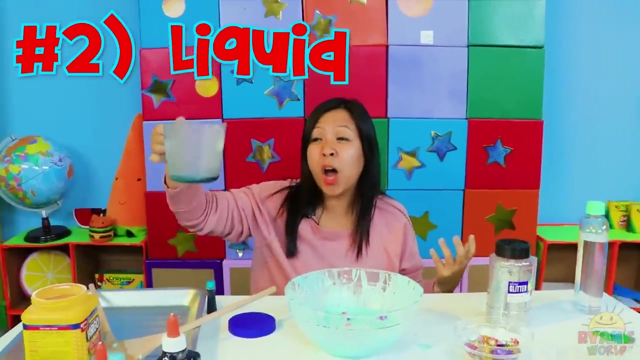 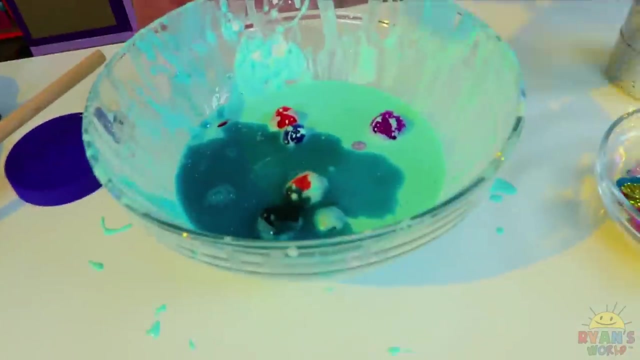 recap, the three states of matter are solid, which has a definite volume and a definite shape, like this ball is a circle- oh sorry, Gus. second is a liquid, like this water here, a definite volume but not a definite shape. and the third type of matter is a gas. 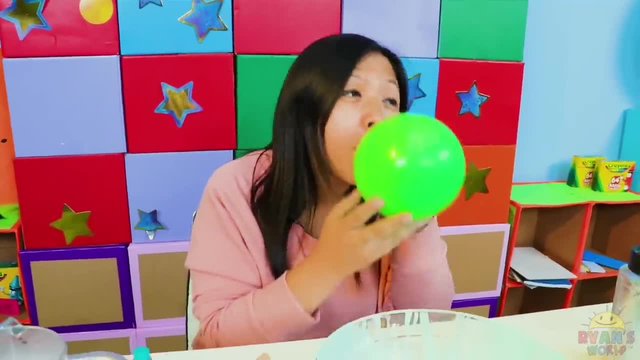 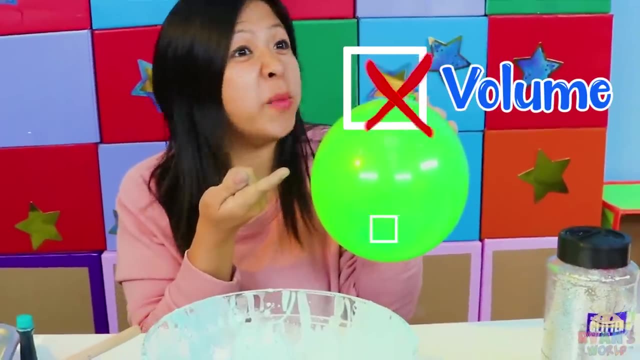 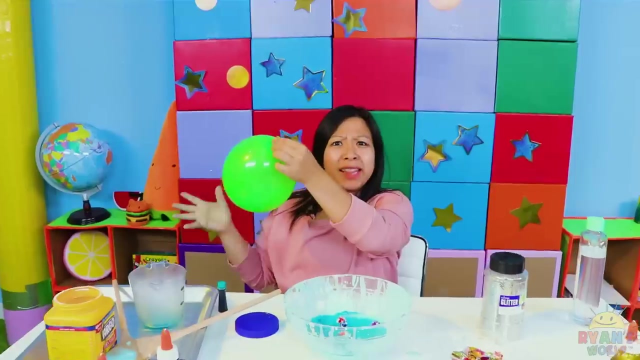 the gas in this balloon does not have a definite volume and does not have a definite shape. the gas that it was in my mouth now is inside this balloon. let the gas in the balloon go, and now the gas will spread all over the balloon. the air is flowing all over the balloon. 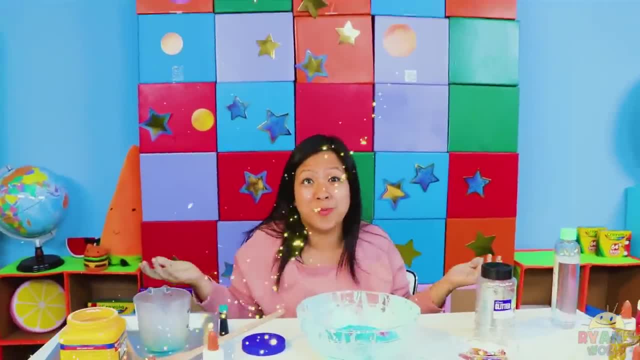 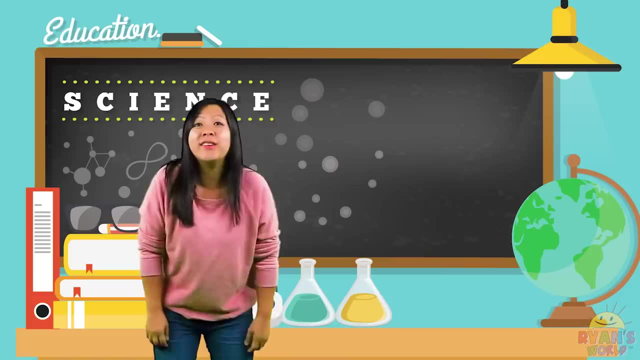 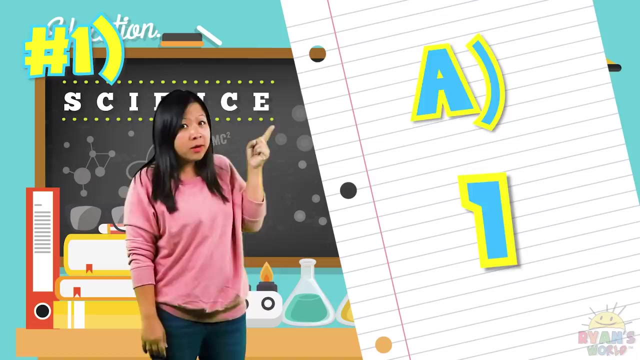 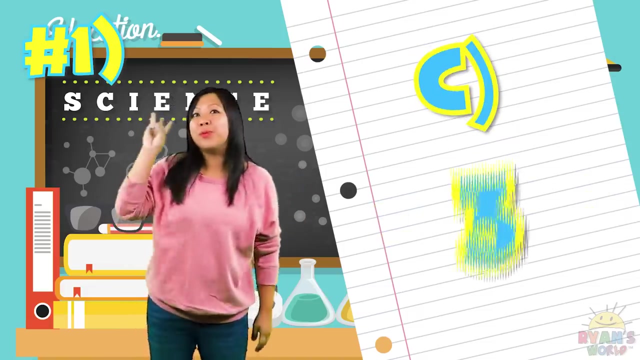 now the gas will spread all over the balloon spread and takes the shape of a room. so now that we learned all about solid liquid and gas, how about we take a test? question number one: how many states of matter are there? is it a- one state the matter, or is it b- a million states of matter, or the c- three states of matter? 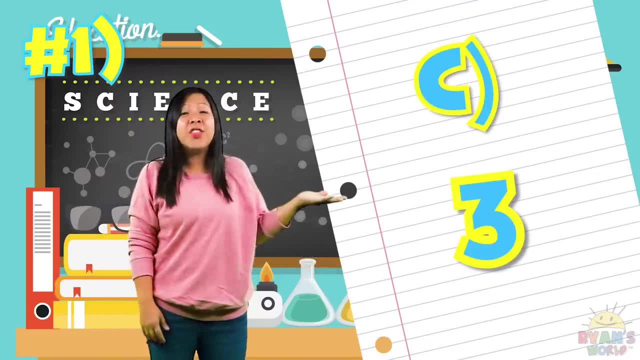 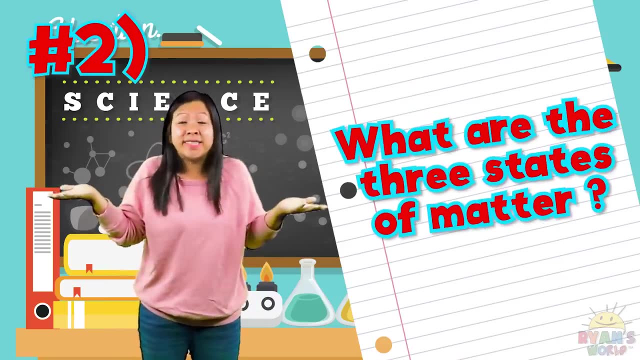 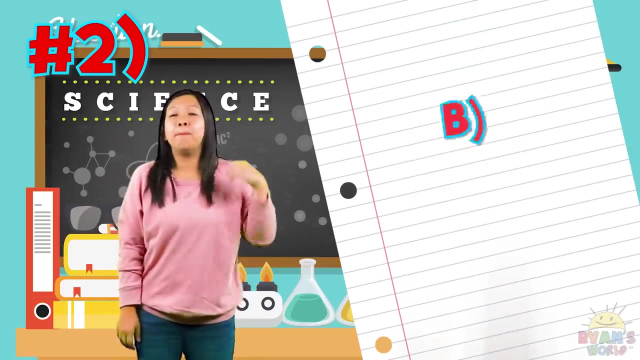 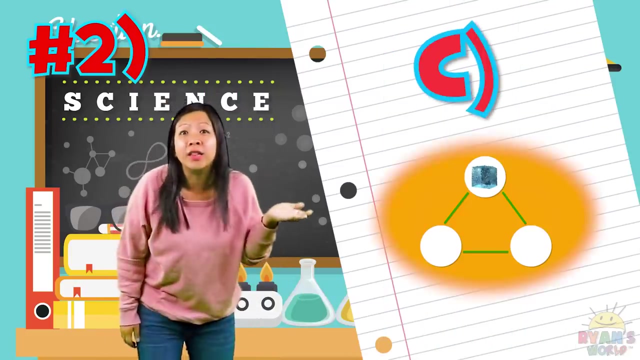 that's right. the answer is c. there are three states of matter. question number two: what are the three states of matter? is it a- lion, bears and tigers, or is it b- sun, moon and stars, or is it c- solid liquid and gas? well, that's right. 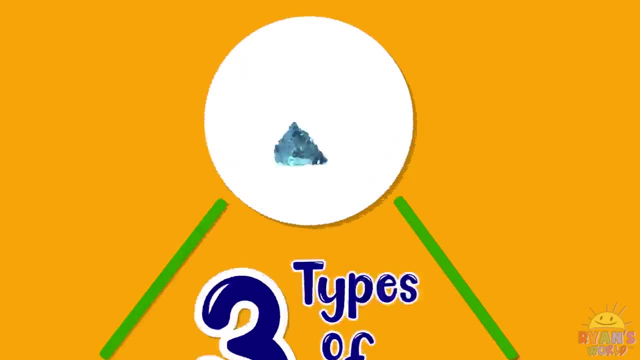 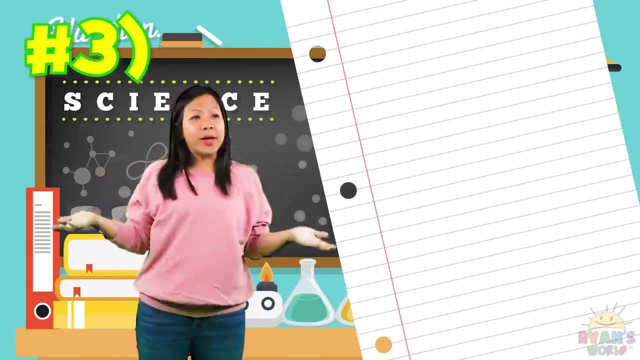 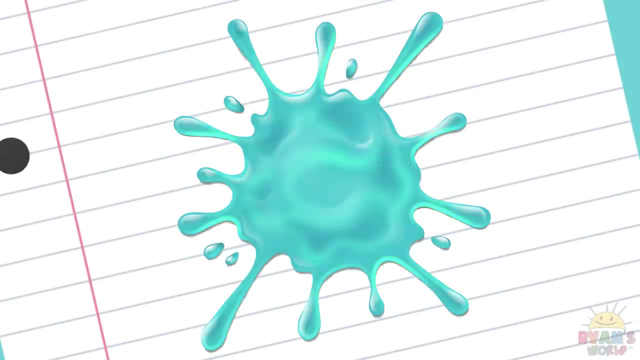 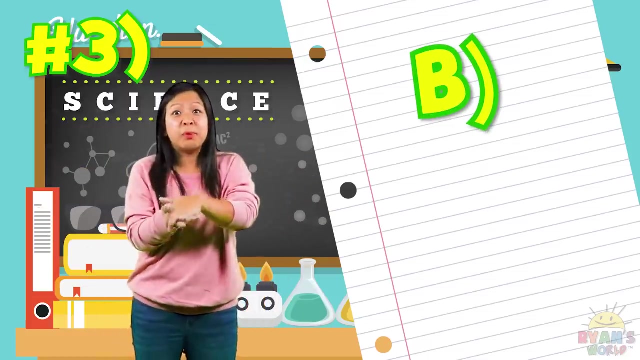 right, it is c. the three states of matter are solid, liquid and gas. question number three: what can a non-newtonian liquid do? is it a, it can change color, or is it b- it can change its viscosity if a strong force is applied. or is it c- it can sing? 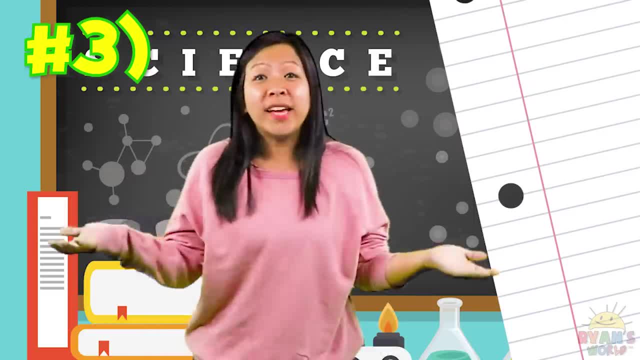 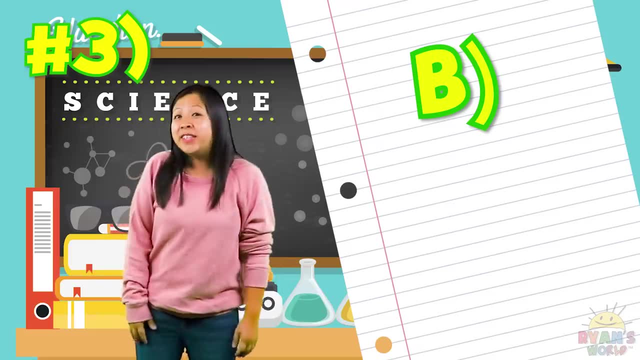 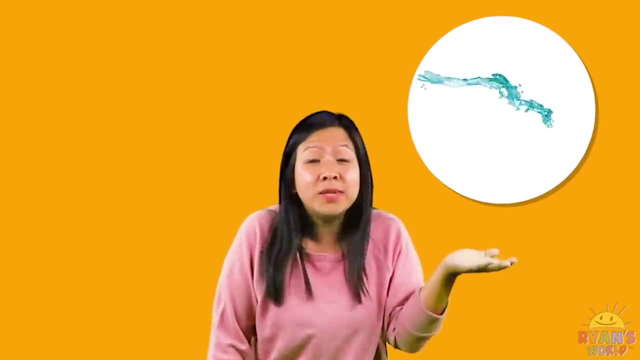 oh, did you guys guess the answer? that's right. a non-newtonian liquid is c. it can change its viscosity if a force is applied, so sometime it could be a liquid or sometime it could be a solid. so now that we learned so much about solid liquid and gas, let's go back and tell ryan: let's go. 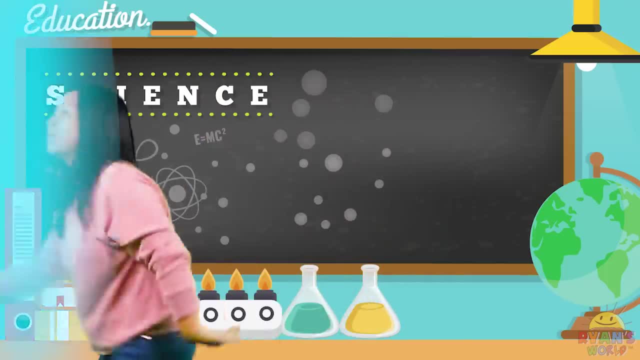 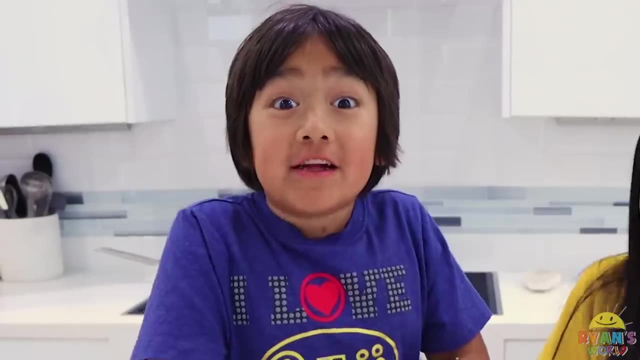 so there it is. that's why uber has been ryan's favorite and sadly he's on the other side of the planet. so there he is. Black is a liquid and a solid at the same time. Wow, that's so cool. I didn't know it could be a liquid and a solid.